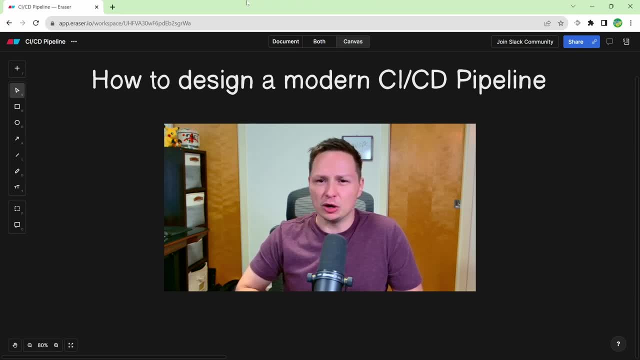 Hey everyone, today we're going to have a look at how you can design a modern CICD pipeline. So if you're a software engineer, a DevOps engineer, if you're designing a pipeline, this is going to be a good video for you. So in this video I'm going to go over the general 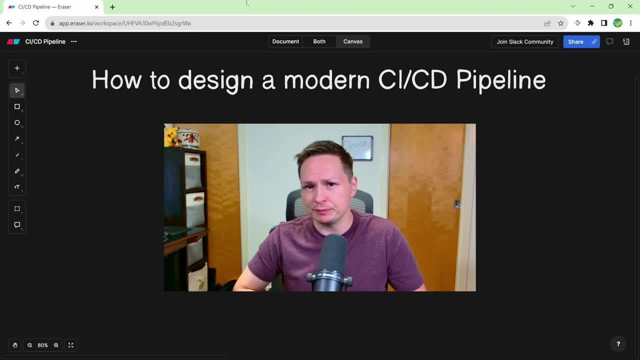 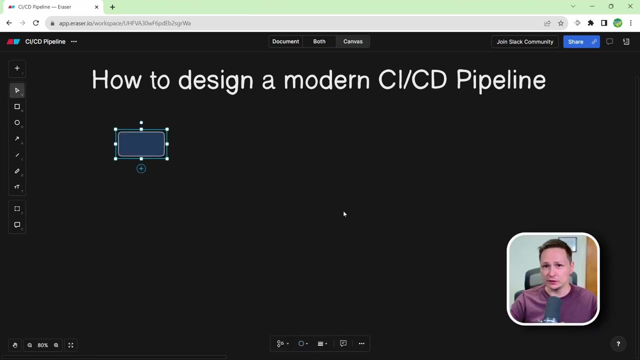 concepts of designing a modern CICD pipeline. So, no matter what industry you're in, no matter what type of application you're creating, this should all be applicable to you. So let's go ahead and start diagramming this out. So, basically, every pipeline is going to start with what's known as. 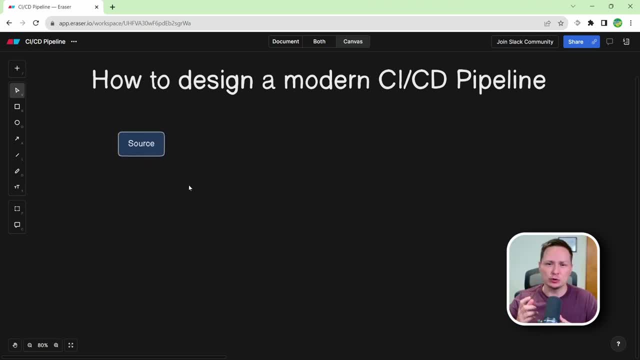 the source stage, And the source stage is a pretty simple one to understand. Basically, this is just getting your code from your code repository, such as something like GitHub or Bitbucket. Now there are a few steps that I like to include in my source pipeline. So the first. 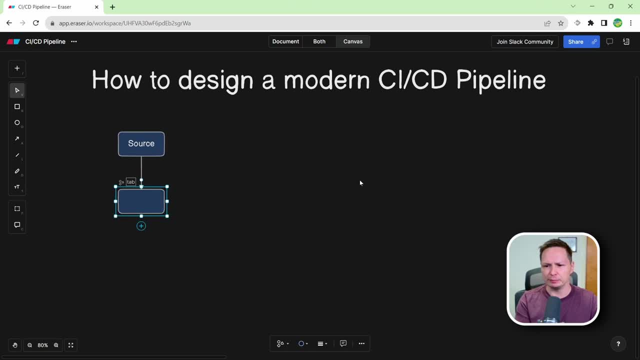 thing I like to define in my source stage is just having some basic branch protectors. And when I say branch protection I just mean like simple rules where you have to have some sort of PR review before a developer can merge their code to the main branch. So you never want 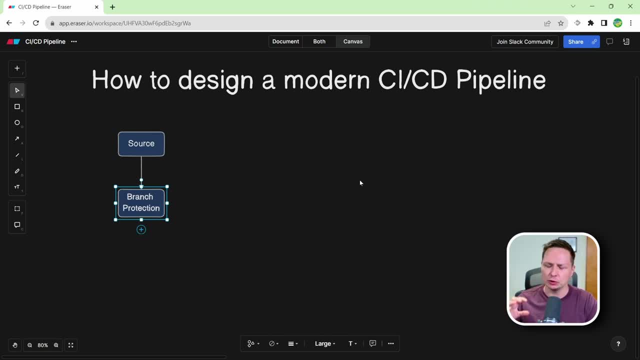 it so your developers can just push up to the main branch. You want some branch protection. you want some sort of PR process. So that's the first thing. The next thing I like to implement at the source stage is linting, So linting, if you don't know about it. 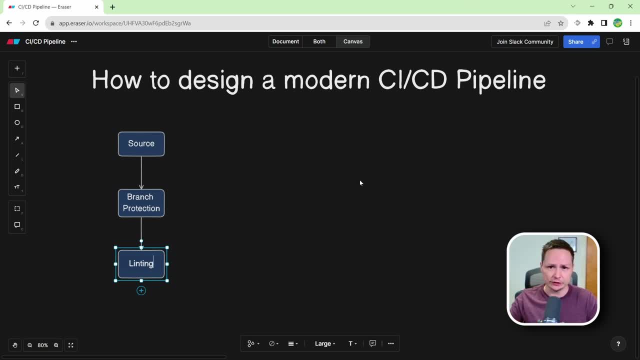 basically, this is just checking your code for syntax errors. There's many different linters out there. Basically every single programming language, YAML document, any type of configuration language, has a linting program that you can implement into your CICD pipeline. So one. 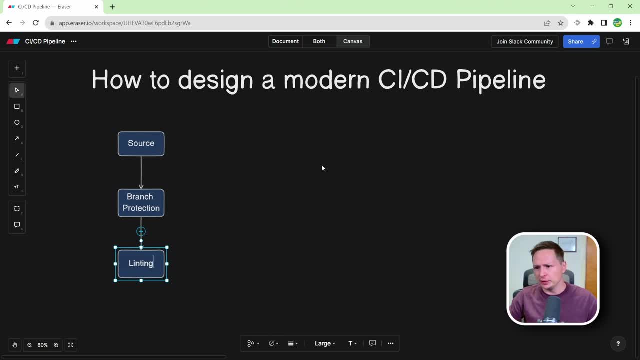 practical example of how I would implement this into a pipeline is: I would just have a GitHub action and it would give either a passing or failed status check if the linting checks failed And if it has a failing status check, the PR can't be merged until the linting problem has been. 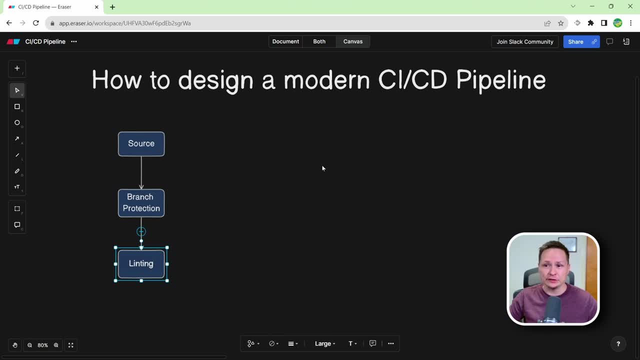 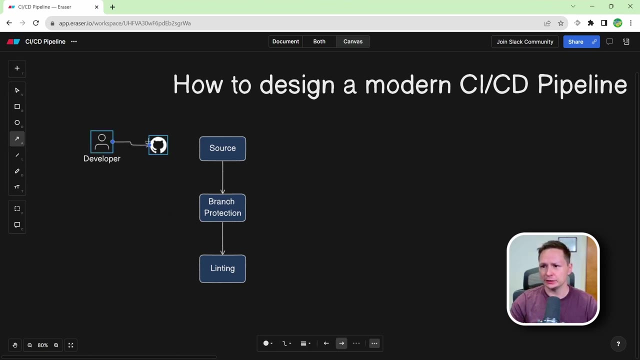 resolved. Now one other thing I like to do. it actually happens before the source stage and it actually happens before the developer can even commit his code. So let me explain this with the diagramming here. So let's add a developer, And this developer is going to commit their code to. 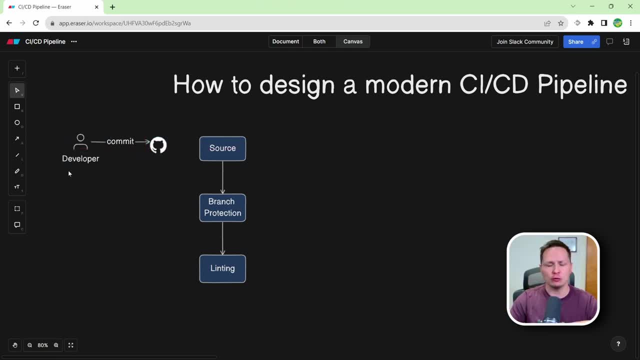 GitHub. But one thing I like to do is have what's known as a pre-commit hook that's built in to the developer's IDE. that will actually run these linting checks locally on their machine before it even lets them make the commit. So what we have here so far is the developer goes. 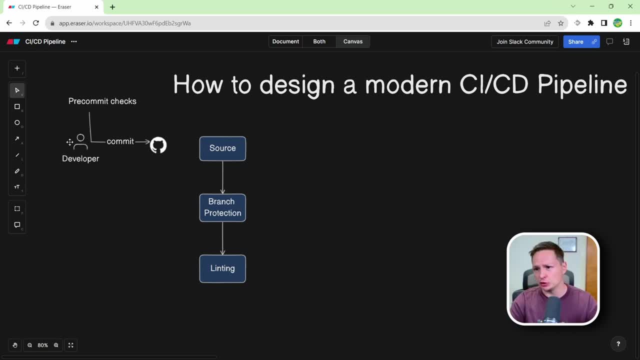 to write his code before he can actually commit and push it to GitHub. They're going to have to pass their local pre-commit checks And then, once it gets to your source control repository, then that's what triggers the source stage. Then we have our PR checks. 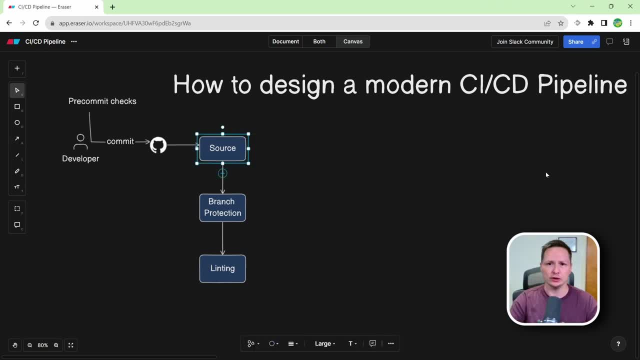 the linting checks and then we can move on to what's known as the build stage. So with the build stage, this is all about getting an artifact that you can then test and then release. So the first part of the build stage is actually compiling your code and building your container images. If 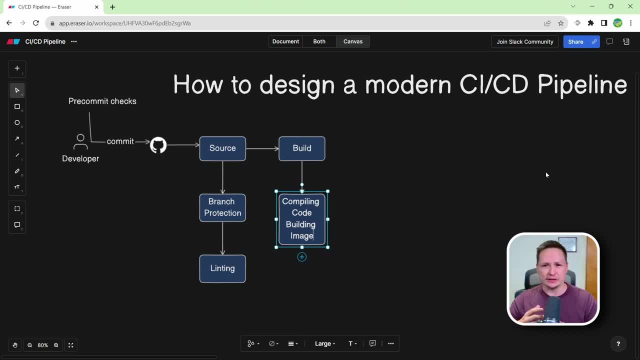 you're using a technology like Docker, which, if this is a modern technology, you're going to have to run CI CD pipeline, you definitely are creating container images of your application. Now, actually, the order of this: you can either compile your code first and then build the image. 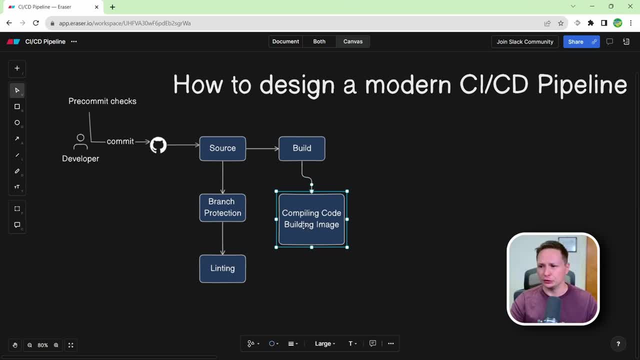 or you can build the image first and then compile your code within it. So usually actually, how I like to do this is I will actually build my container images first using my Docker file and then I'll actually compile the code within my Docker image. So this is all personal preference. 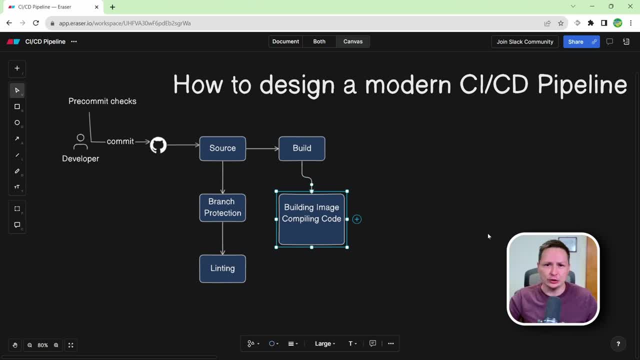 how you do it. So all that really matters is you have your code built and you have a container image that you can start using to run your unit tests. So our output here is going to be a container image, And that container image we're going to use to actually run our unit tests on. So unit tests are basically 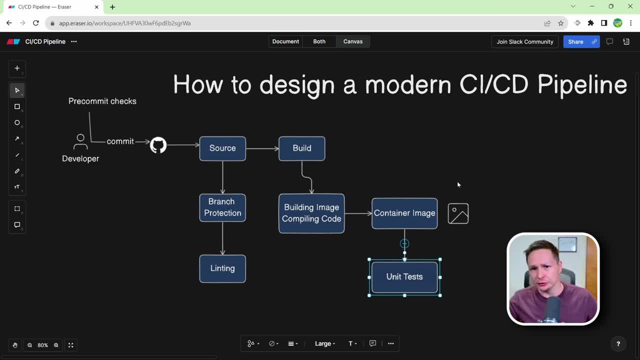 just a way to test the basics of your code. So every time a developer submits new code or a new function or anything like that, they should be building unit tests And then those unit tests run during this stage of the pipeline. So if you had a calculator app, basically a unit test would be: does five plus five equal 10?? Does? 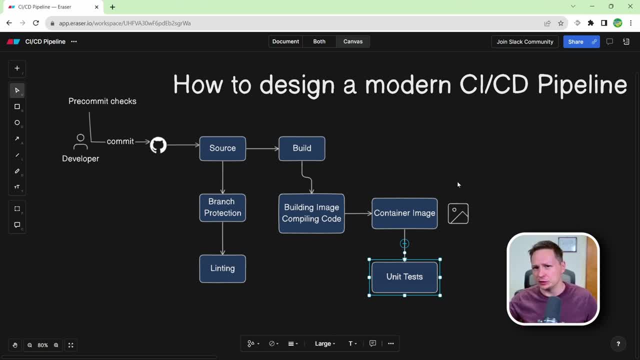 five minus three equal two. you can think of a unit test to be just simple checks like that. Now, once your unit tests are done, one other thing that I like to do in the build stage is to check for code coverage. So let's add a node here. 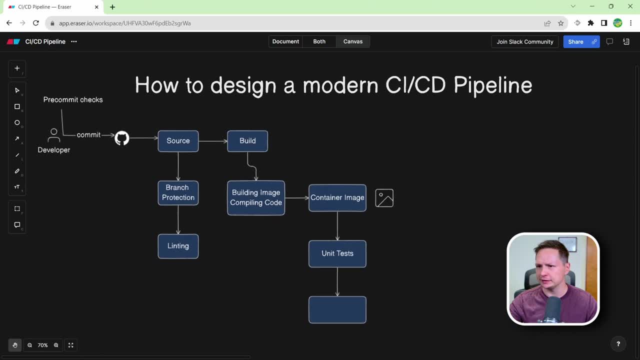 Scroll over, maybe zoom out a little bit and go code coverage check, And usually I like to check for about 80 to 90% And the percentage is really going to depend on the organization and the type of application. Now, if you're not familiar with what code coverage is, basically, it's just. 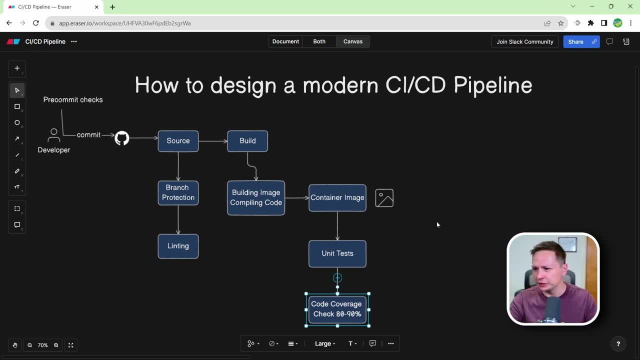 checking your code to make sure that your developers are putting in unit tests. So if you have unit tests for 90% of your code, then you would have a code coverage of 90%. If you only had unit tests for 80% of your code, then your code coverage would be 80%. So this is one thing. 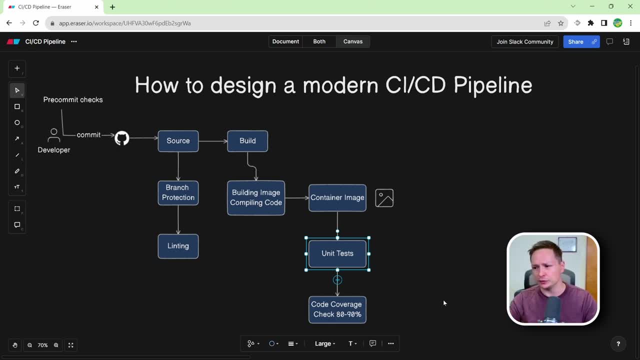 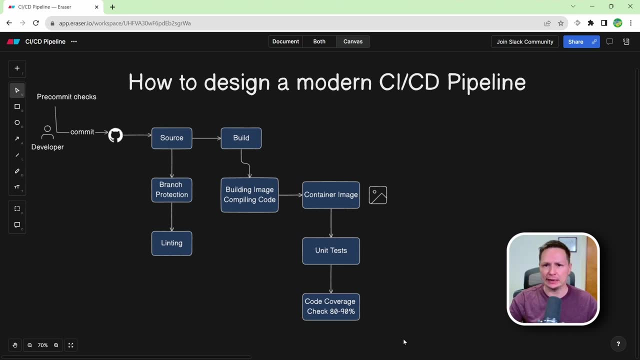 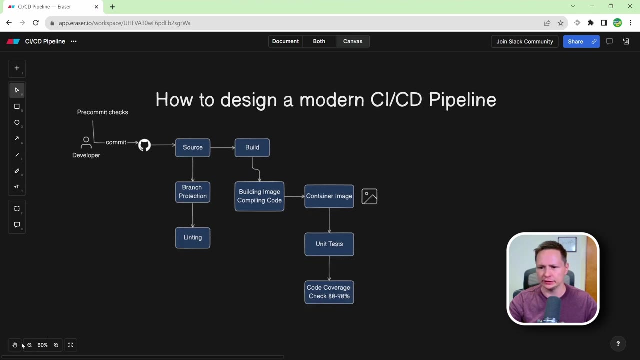 that I like to gate. if the code coverage ever falls below a certain percentage, then I like to fail the pipeline there. Now, once your build stage is done, it's time to move on to the testing stage, where the real testing happens. So I'm going to actually just zoom out here a little. 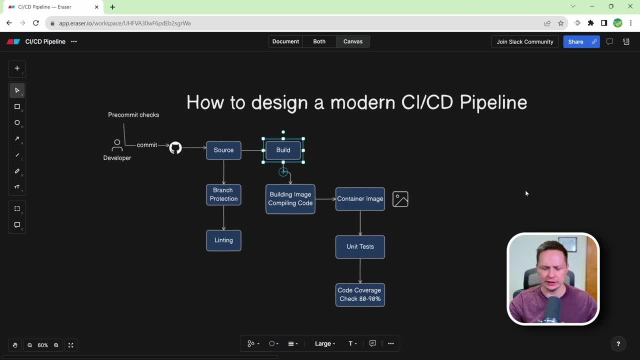 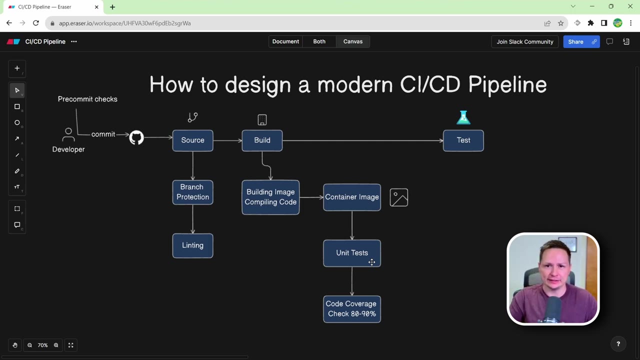 bit And let's add another stage to our pipeline. So we'll add the test stage And let's go ahead and add some images here to make this diagram a little nicer, Alright, so like I said in the test stage, this is where the real heavy testing happens. So in the build stage I do the simple testing, like: 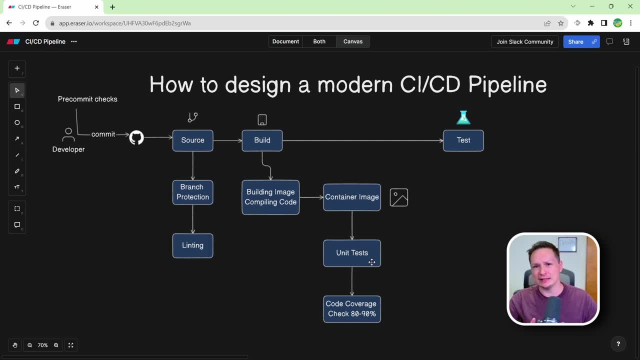 the unit tests and the code coverage checks. But in the test stage we want to actually test out the integration tests, So we'll add this here. So basically, what an integration test does is it's going to test the functionality of your application. So if we had sort of like a social 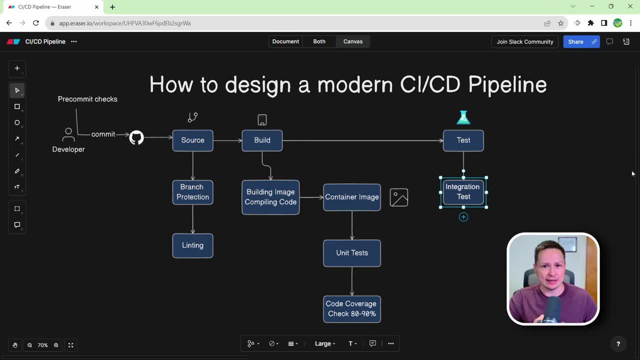 media application. one of the functions that we may test is: can a user post a new message? Can someone comment on that message? Can they upload photos? Can they delete a photo? What happens if this happens? This is where all those complicated tests happen. This is where all those complicated 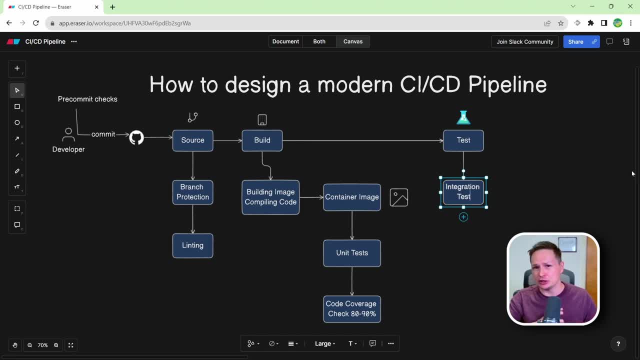 tests happen. This is where all those complicated tests happen. This is where all those complicated tests start to run And your functionality of your application gets fully tested. So this is actually one of the longer stages of your pipeline, because running all those integrated tests does. 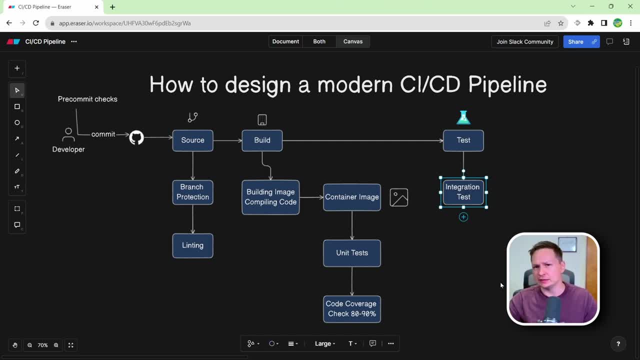 take a little bit of time Now. one other thing to keep in mind here is, if you're building an image and then testing a container for a microservice, that microservice probably has a lot of other dependencies. it probably depends on a lot of other microservices in your infrastructure. it 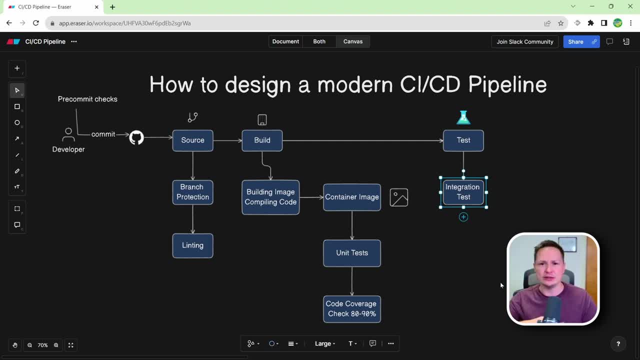 probably depends on your databases, So you have to make sure that you're able to bring up an integrated testing environment. Now, using something like Docker. compose can do this for you, But you can also run this in a full testing environment in a Kubernetes cluster. this is really going to depend on the 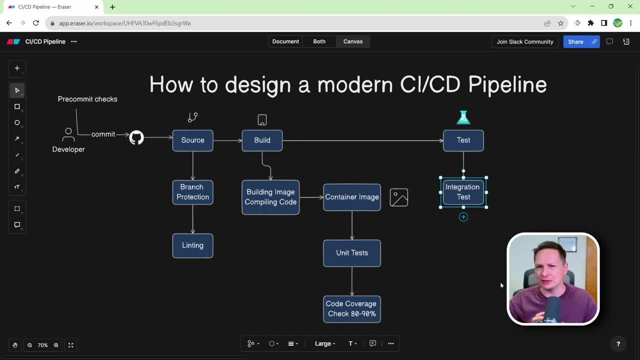 organization, their testing suites that they need to run and the type of application. So I like to leave this one a little bit open for how you actually integrate it into your pipeline. So that's all I wanted to mention about the testing stage. Let's now move on to the final stage of the CI CD pipeline, which is the 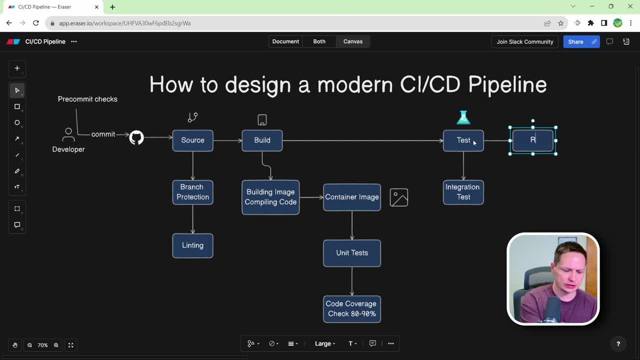 release stage. So the next stage here is release. This stage is all about releasing your application so your servers can start using it. So what happens in the release stage? Well, this is usually when you ship your image to registry. So let's get ECR registry here. 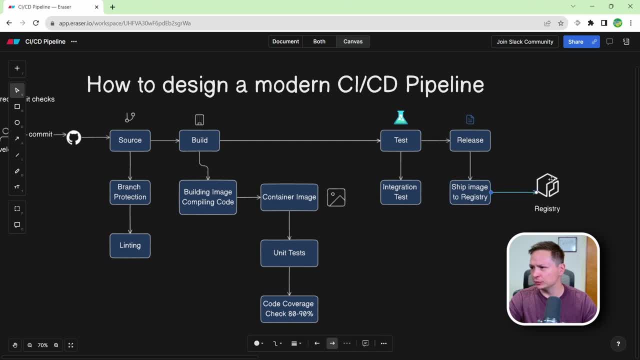 And point this to our registry. So when your image is available on your registry, that's when all your other environments can start pulling it down and running your application. So this is going to be something like a qa environment, So your qa engineers can run extra. 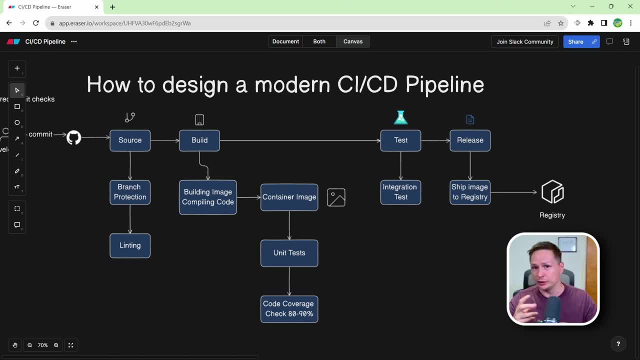 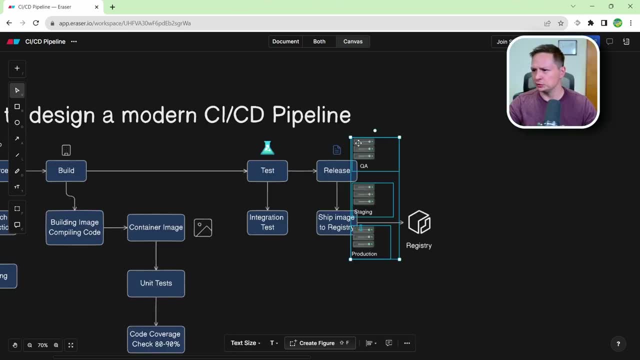 tests to your application. This might be a pre production environment, such as a staging environment as well, Your production environment. So let's plug those in here, So all these different environments can get the image from the registry. now Let's scroll up here and have a look at this whole thing.